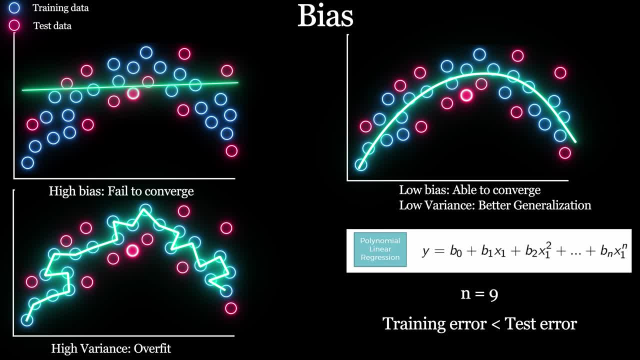 but when you use the same model to perform on test dataset, the error will be too high. So this happens when a model has high variance. But if you tune the degree of polynomial again a little bit then you can have a model with low variance. 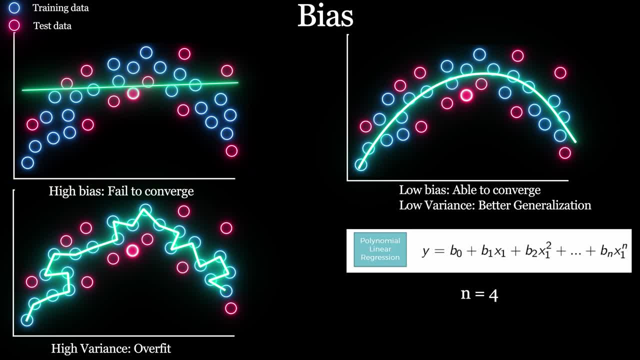 Now, as far as we saw, a model with high bias makes very simplistic assumption and unfits the data, Whereas a model with high variance capture noise and overfits the data. But when a model has low bias and low variance it adapts very well on the dataset. 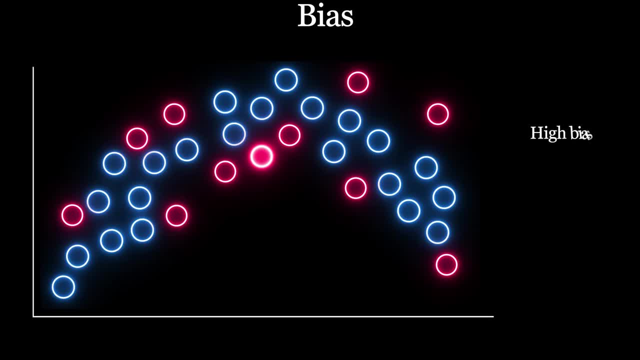 And one more thing you may have noticed Is in case of high bias, the model try to approximate target function, like this, Which is very similar case like if a model has low variance And when a model has high variance tries to approximate target function, then the case is similar, like model has very low bias. 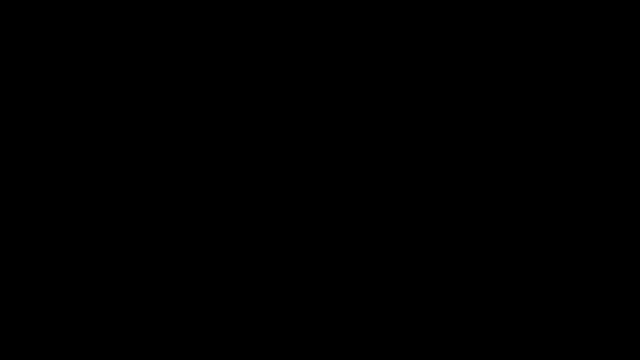 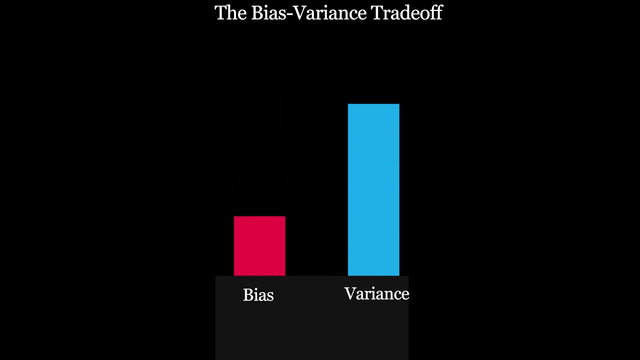 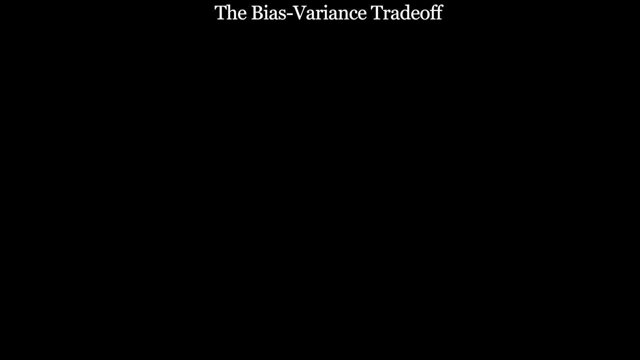 And this relationship between bias and variance brings us to a famous trade off called the bias variance trade off, Where, if you try to decrease one, the other will start increasing and, as we already saw, that a model with low bias and low variance performs well. So, to conclude, we can have four types of cases: while training, a machine learning model. 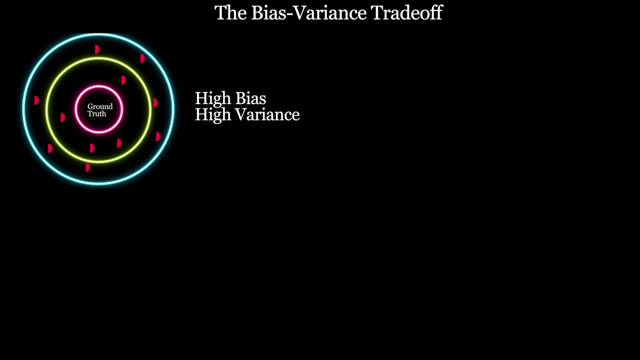 A model with high bias as well as high variance. High bias will not let the model to adapt training data, which will lead to high average training error, and high variance will make it very sensitive with respect to change in data, which lead to inconsistency in prediction. 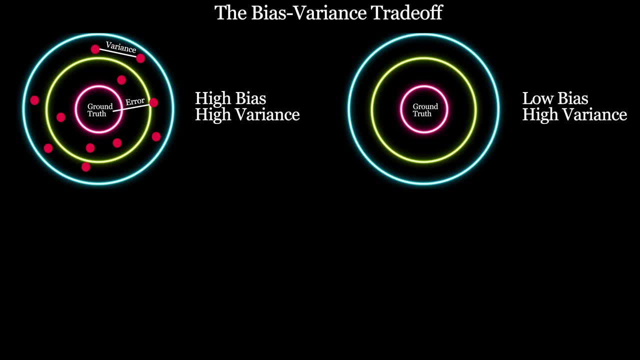 Now second case: A model with low bias and high variance. Due to low bias, the model will adapt training data and you will get low average training error, but you will still see inconsistency in prediction. That is, high average error on test dataset due to high variance. 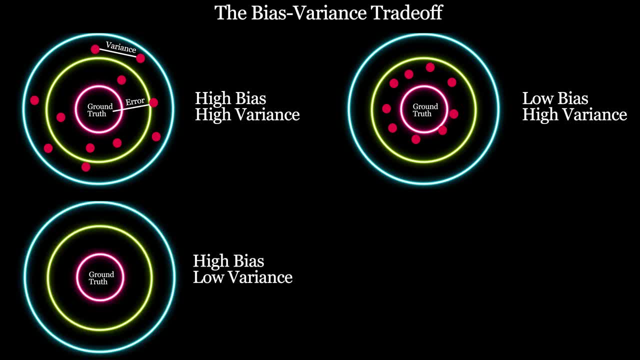 Third case: A model with high bias but low variance. As you know, high bias will increase training error but the model will less inconsistent in prediction due to low variance. And the fourth one is A model with low bias and low variance Because it adapts very well on training dataset due to low bias and become consistent. and